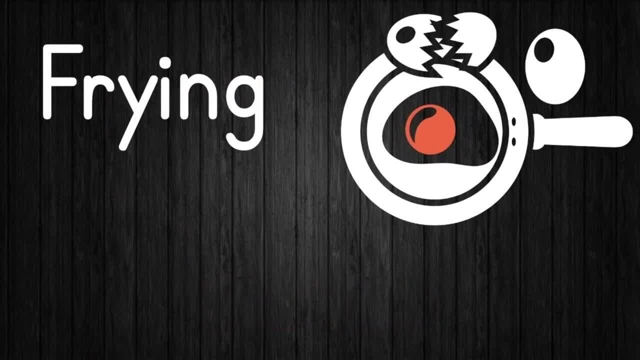 over relatively high heat. The common recipes for frying are fried egg, fried fish or any dish that is turned once or twice during cooking using tongs or a spatula. Sautéing is a French word for jumped or bounced. 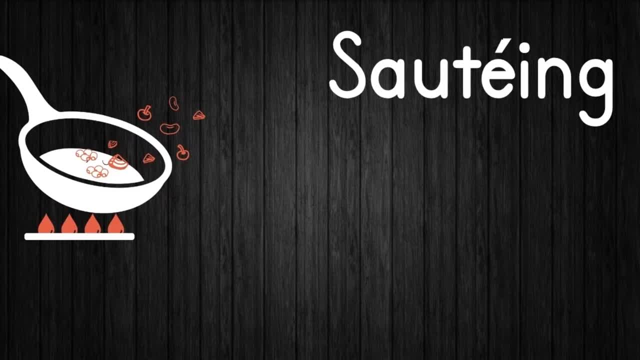 Frying is similar to frying. the ingredients are also cooked in an oil or fat in a shallow pan over high heat, except that the foods are cooked by tossing in the pan. The common recipes for sautéing are sautéed vegetables or sautéed shrimp. 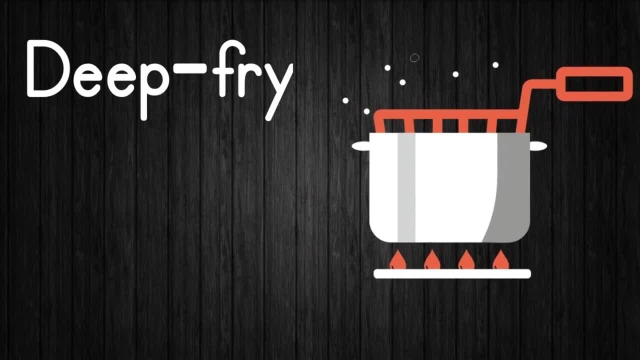 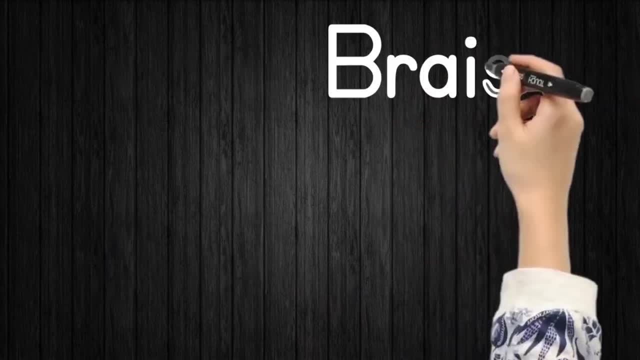 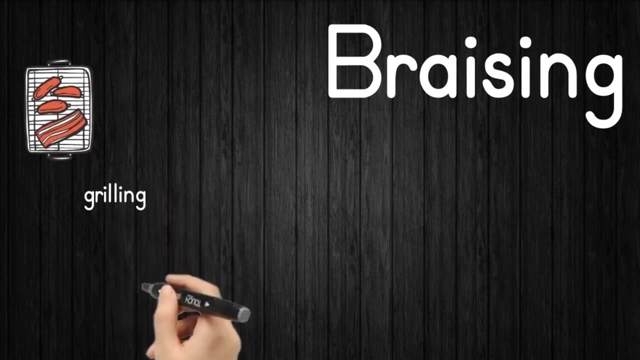 Deep fry is a cooking method where foods are completely submerged in an oil or fat. The common recipes are French fries and fried chicken. Braising is a cooking method using both dry and wet heats. First, the food is cooked at a high temperature by any means like grilling, roasting or broiling. 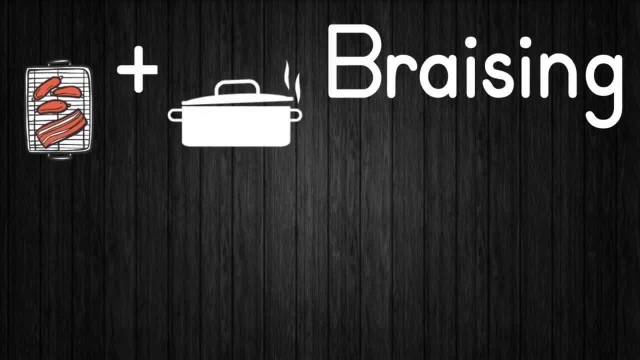 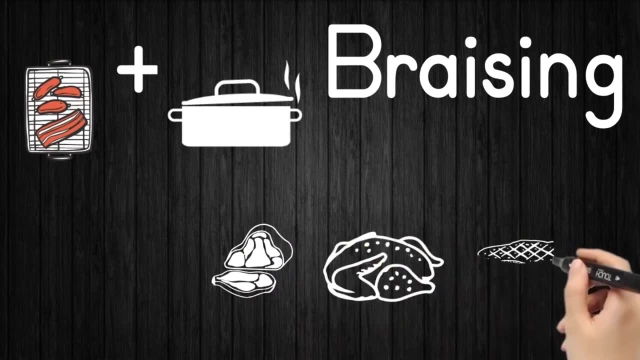 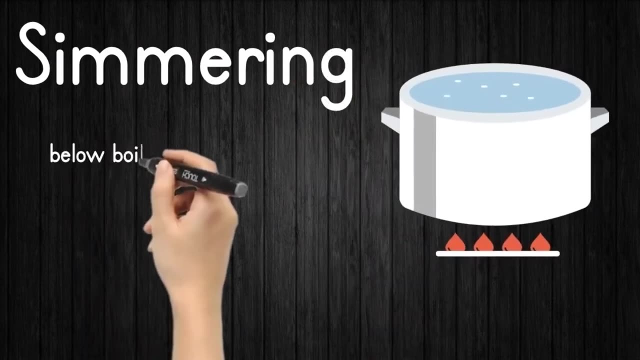 followed by the moist cooking method in a covered pot at a lower temperature, while sitting in some amount of flavored liquid. The common recipes of braising are braised beef, braised chicken and braised pork. Simmering refers to the cooking method in a liquid that is just below the boiling point. 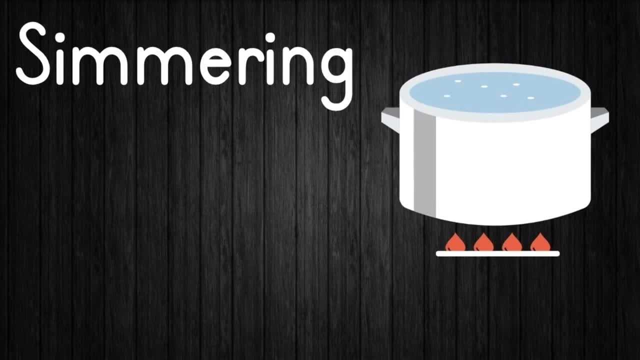 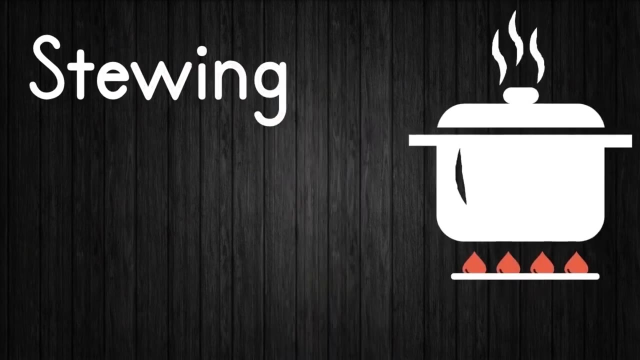 With simmering you'll see bubbles forming and gently rising to the surface of the water, and the water is not at a full roll. Simmering is the most common moist cooking method, like simmering stocks and soups, to cooking vegetables. Stewing is a slow cooking method in a closed pan where the meat or vegetables are cut into. 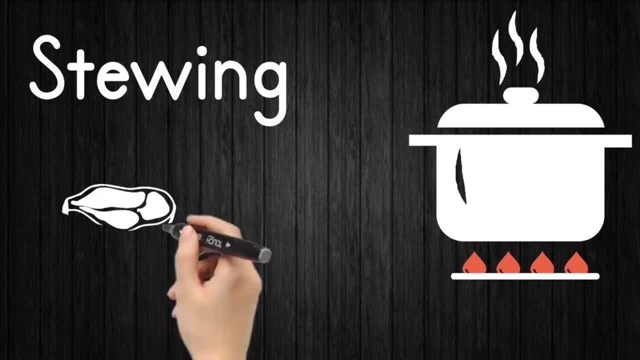 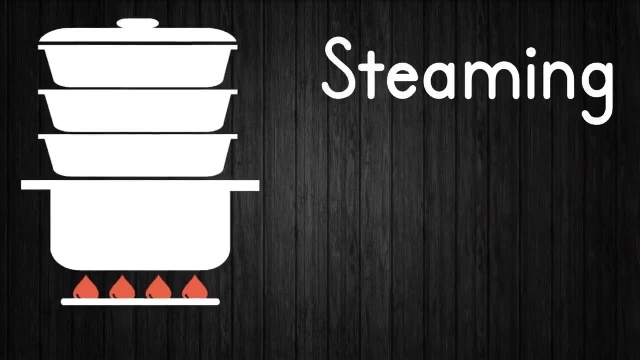 smaller pieces and submerge in the liquid. The common recipes of stews are beef stew or bean stew. Steaming is a cooking method where the heat of moist is used. This method is done by continuously boiling the water, causing it to be too hot and too. 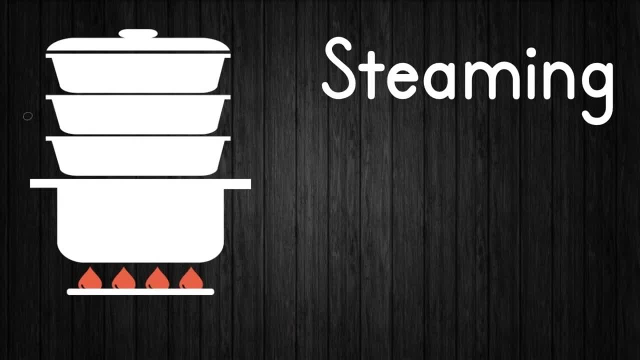 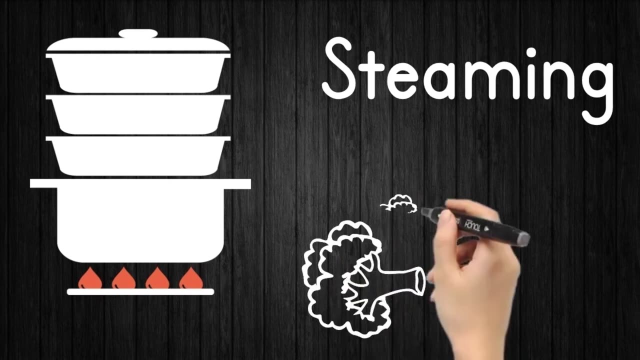 causing it to vaporize into steam. This steam then carries heat to the nearby food, thus cooking the food. The food is kept separate from the boiling water but has direct contact with the steam, resulting in a moist texture to the food. The most common recipe for steaming is steamed broccoli or 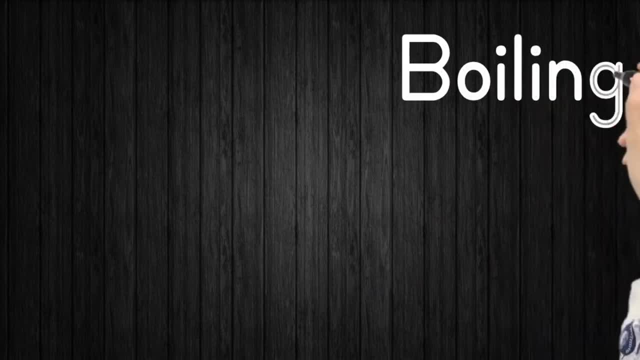 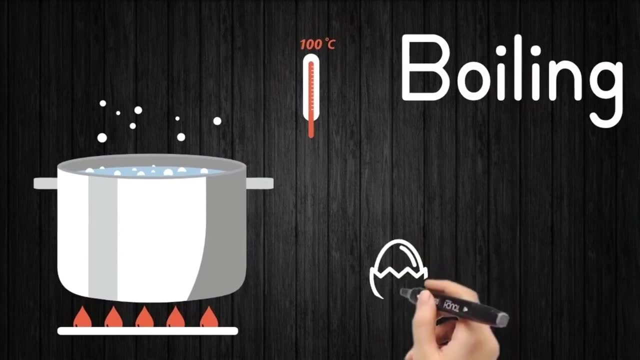 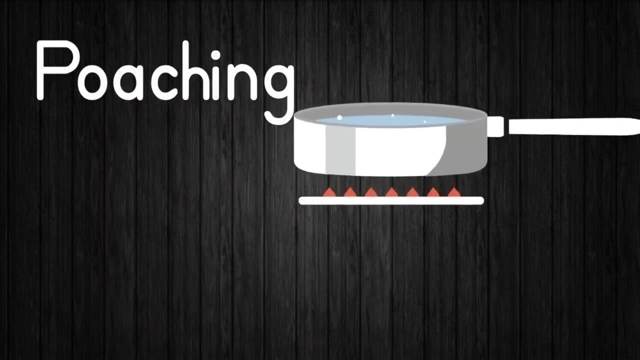 steamed fish. Boiling is a wet cooking method where ingredients are cooked in water at 100 degrees Celsius. The most common recipe for boiling is boiled egg or boiled potatoes. Poaching is a cooking method that involves cooking by submerging food in a liquid. 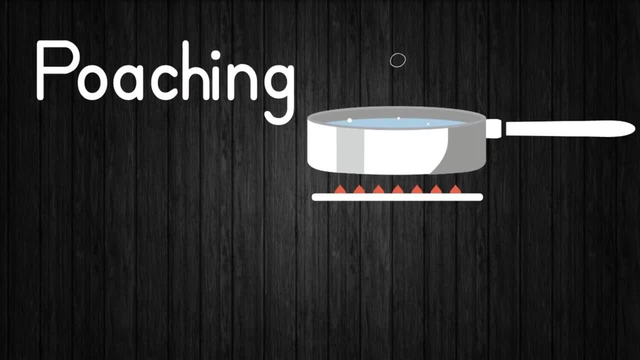 Poaching is different from simmering and boiling because it uses relatively low heat. There should be few to no bubbles in the water. This is suitable for delicate foods like eggs, fish or fruits that would be disturbed or destroyed by aggressive bubbles. The most common recipe for boiling is steamed broccoli or steamed fish. This is suitable for 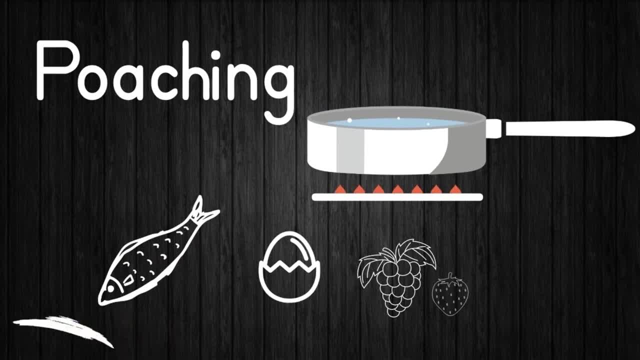 delicate foods like eggs, fish or fruits that would be disturbed or destroyed by aggressive bubbles. The most common recipe for poaching is a poached egg or poached fish. Blanching is a wet cooking method where the ingredient is submerged in boiling water in a 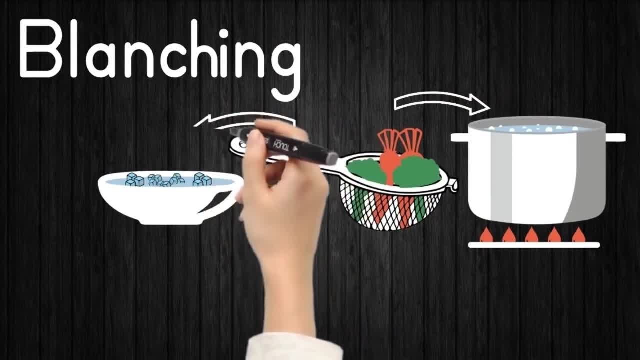 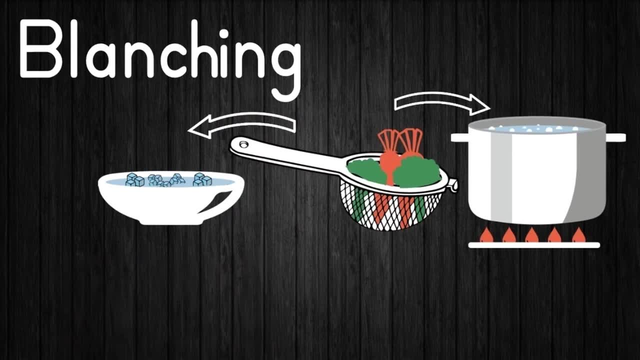 short amount of time and then plunged in water with ice to cool it down quickly. Blanching is commonly used to preserve the color, flavor and nutritional value of the food. The most common recipe for blanching is blanch green beans. This cooking method is mostly used in vegetables. 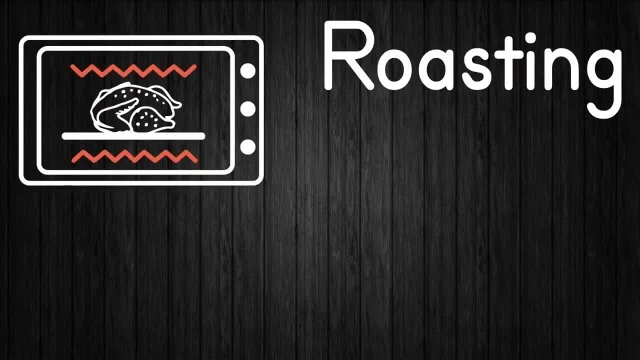 Roasting is a dry heating method. The most common recipe for blanching is blanch green beans. This cooking method is mostly used in vegetables. The most common recipe for blanching is blanch green beans. Baking is a dry heat cooking method where ingredients are cooked in an oven. The hot. 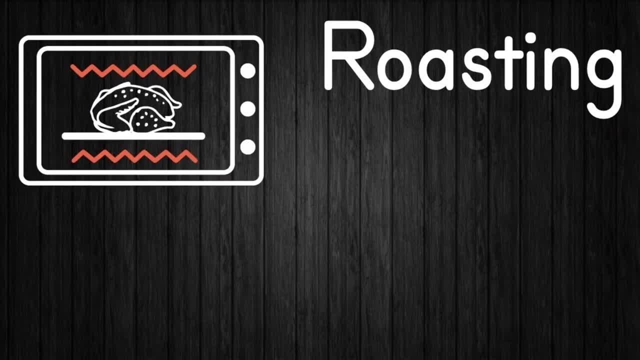 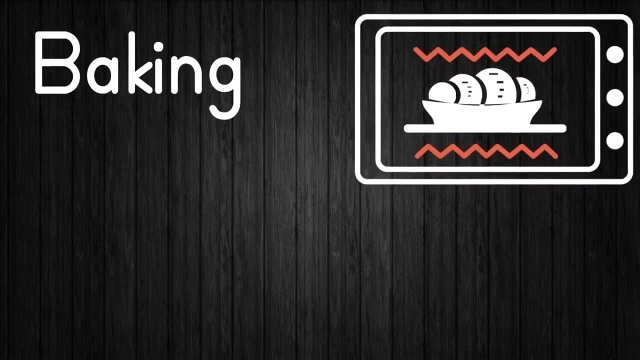 air covers the food, cooking it evenly on all sides. Roasting is suitable for slower cooking of meat in a large serving or whole piece. The most common recipes for roasting are roast chicken or roast potato. Baking is a dry heat cooking method that can be done in an oven or hot stones. 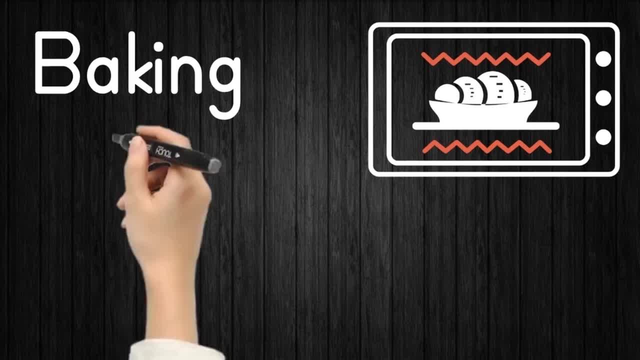 Baking is a dry heat cooking method that can be done in an oven or hot stones. Baking are usually foods prepared from flour or meal derived from some food. Baking is a dry heat cooking method that can be done in an oven or hot stones. Baking is a dry heat cooking method that can be done in an oven or hot stones. 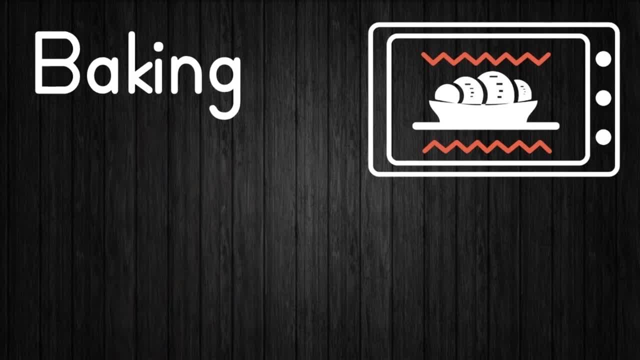 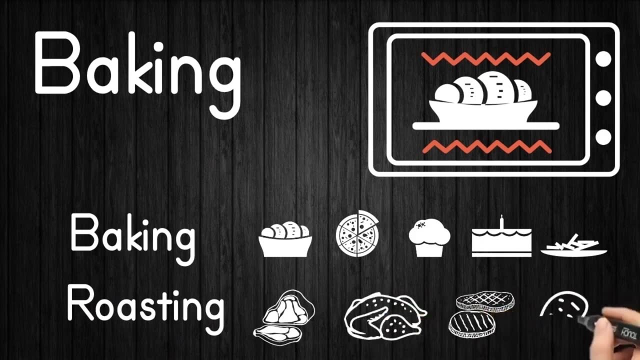 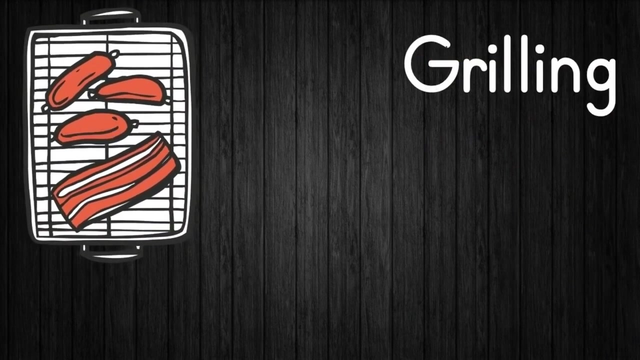